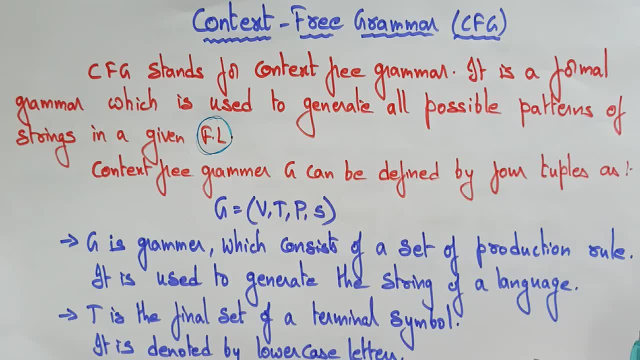 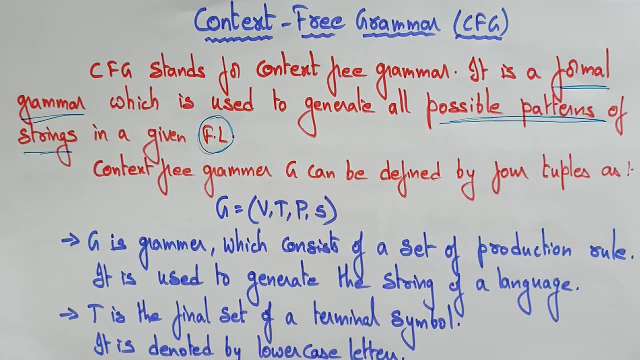 Okay, so actually, what does this context free grammar. We call this as a formal grammar. Why? Why we call this as a formal grammar? Because it is used to generate all possible patterns, whatever the patterns that are available of the string, that different patterns can. it can be generated. It can be represented in leftmost or rightmost, in whatever it may be. Okay, so it can generate all possible patterns of a strings in a given formal language. 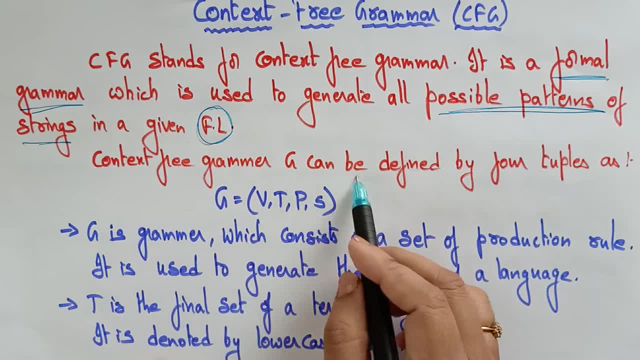 Okay, a context free grammar G can be defined as four tuples. So far, you have seen, whenever we are discussing about the definition, the non deterministic finite automata, deterministic finite automata, okay, whatever we are taking that mille machine and the more machine, everything, every definition is based upon the tuples And that definition is defined by the tuples. Okay, so in the same way, for the context free grammar also, it can be defined as a four tuples. 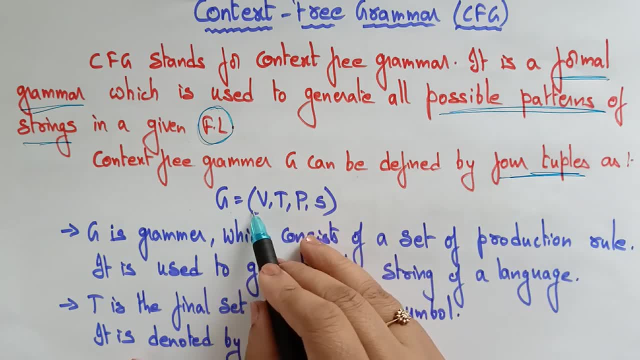 So what are those four tuples? G is equal to VTPS, or you can call it as NTPS also Okay, G is equal to VTPS. So what is this G and what is VTPS? Let's see that. So whenever you ask me about the context free grammar, you can you have to see that it is a formal grammar which is used to generate all possible patterns of a strings in a given formal language. Okay, and it can be defined as a four tuples. That is, graph is equal to VTPS. 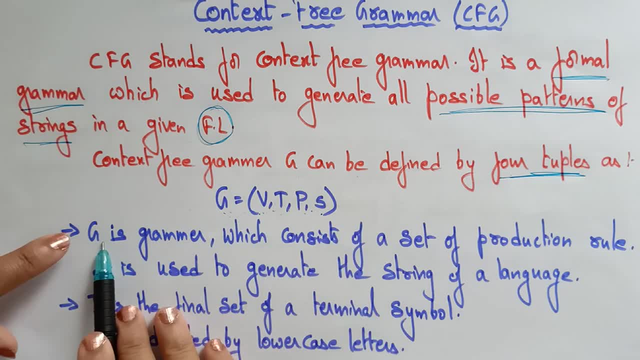 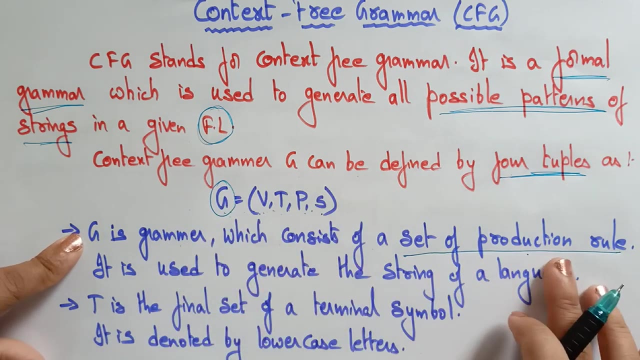 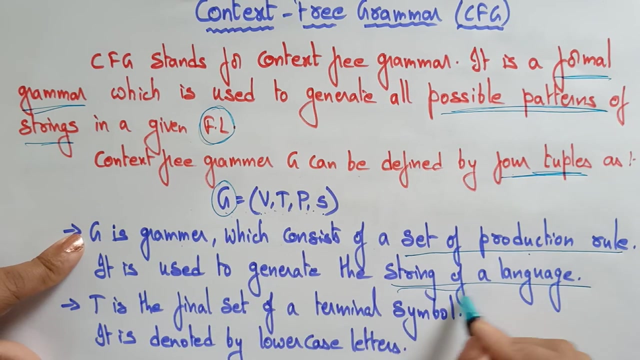 What is G? Sorry, it's a grammar, not graph. G is a grammar which consists of set of production rules. So this G- whatever the G that we are using- it consisting of set of production rules. So what is the use of those rules? It is used to generate the string of a language. So what type of string of language I'm going to get that will be generated by this G grammar? 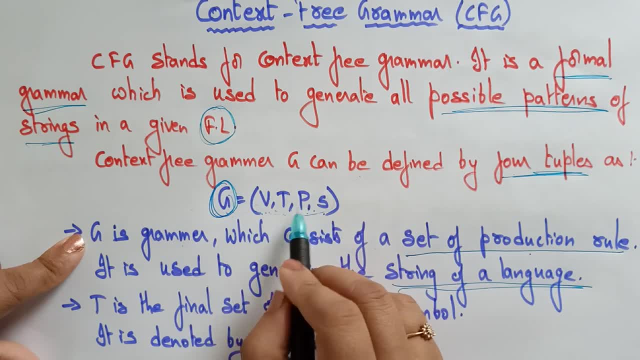 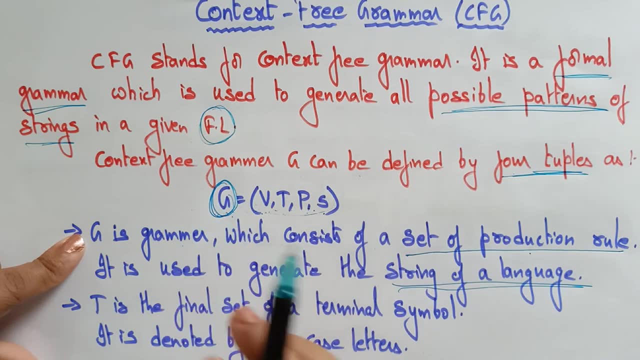 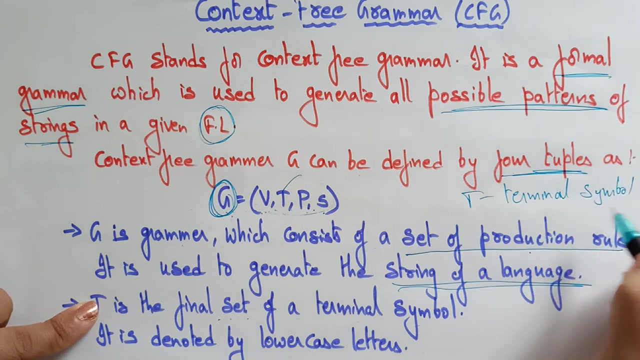 So if you take, or with the help of these VTPS, a grammar is generated, This grammar is used to generate the string of language. Okay, what is the string of a language that I'm using? And coming to the T: T you call it as a final set of terminal symbols. T means terminal. Remember that. Don't confuse Terminal symbols. Terminal symbols means you can take it as a capitals. Okay, so sorry, it is. terminal means lowercase. 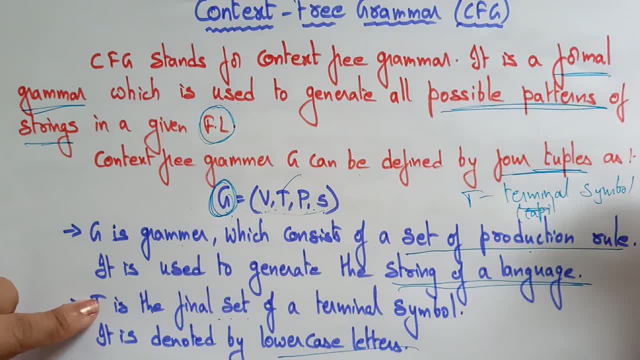 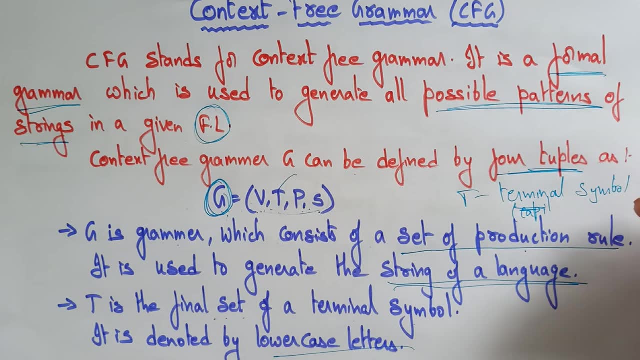 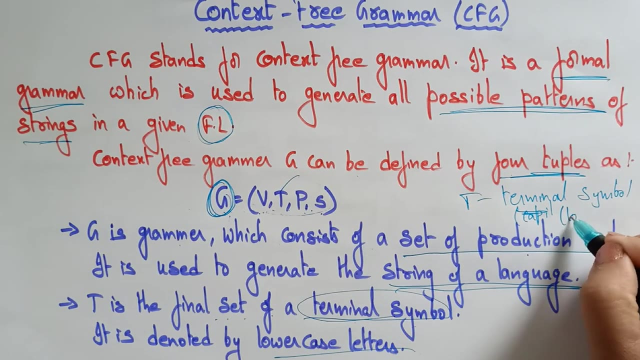 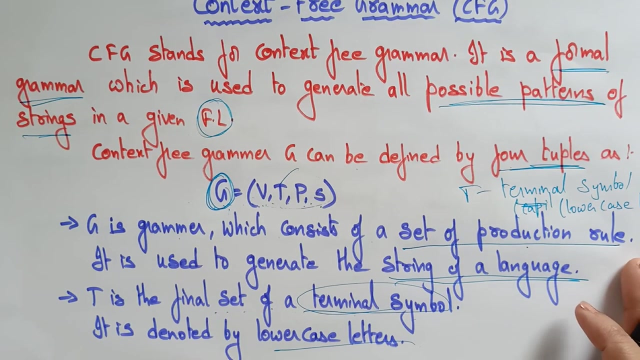 Letters. It's a lowercase letters means the small letters, alphabets, ABC and all the letters. that is lowercase, Okay, not having the least prior lowercase. So T is the final set of terminal symbols. Terminal symbols means you have. you have to remember that lowercase letters, Okay, the lowercase letters, you call it as a terminal symbols. And coming to the P, P is the product or V. 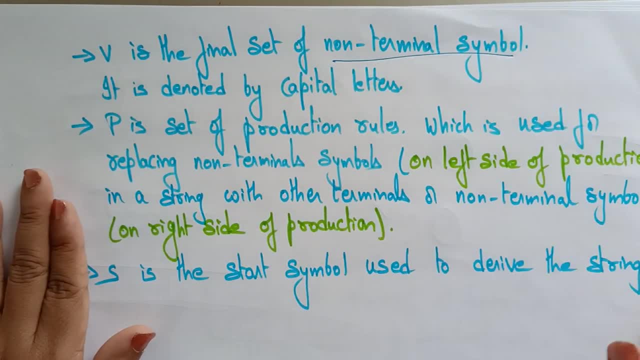 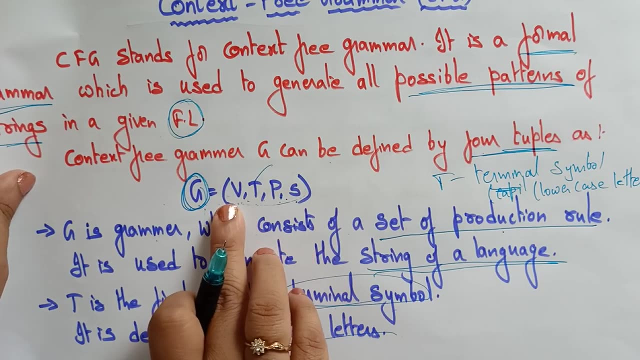 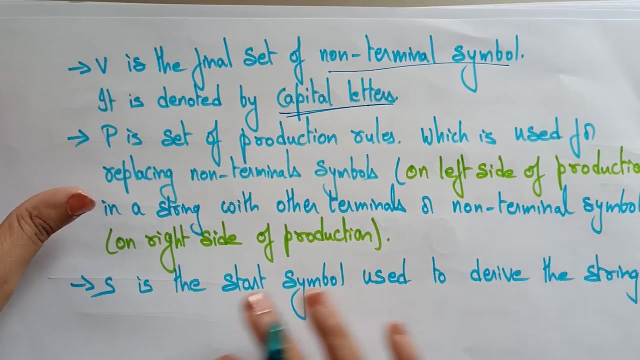 V is the final set of non-terminal symbols I said. I said T is a terminal symbol. T is a terminal symbol. And what about the V? V is a non-terminal symbols. We can represent it. It is denoted by the capital letters. The only difference between that two is V is represented in capital letters. The symbols that are represented in capital letters, Symbols, you call it as a alphabets, or the binary numbers. 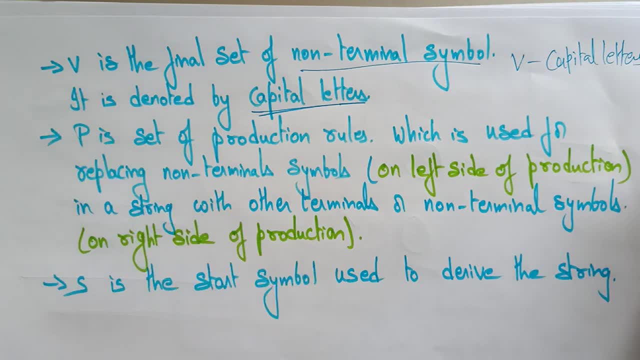 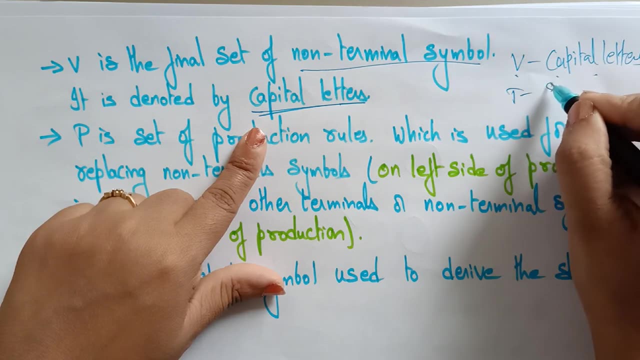 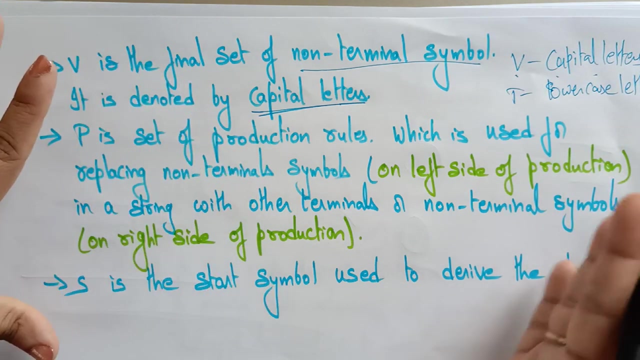 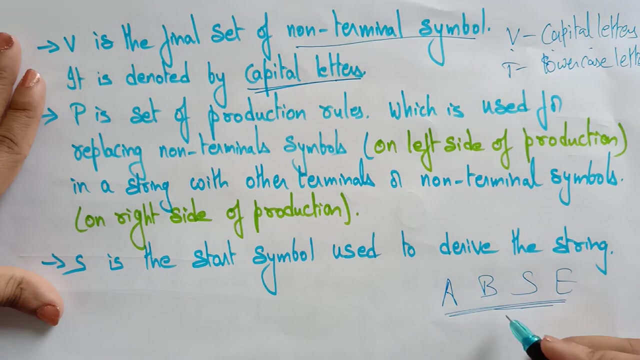 Okay, Or that, or special characters. That is a symbols, Okay. And here V is represented in the capital letters and T is represented in the small letters. That is a lowercase letters. Whenever you see in the production rules, whenever you're seeing like A, B, S, E, So these are called as a non-terminals. Non-terminals, Okay. So these are the sets of V. 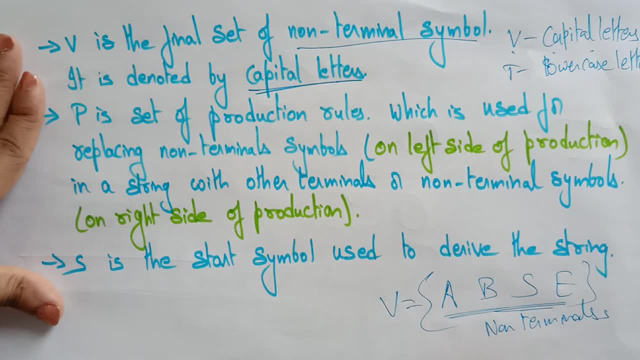 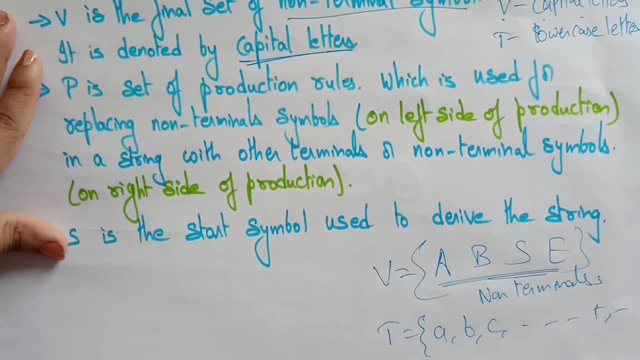 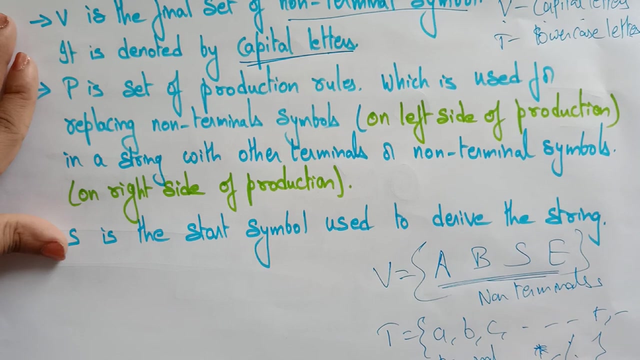 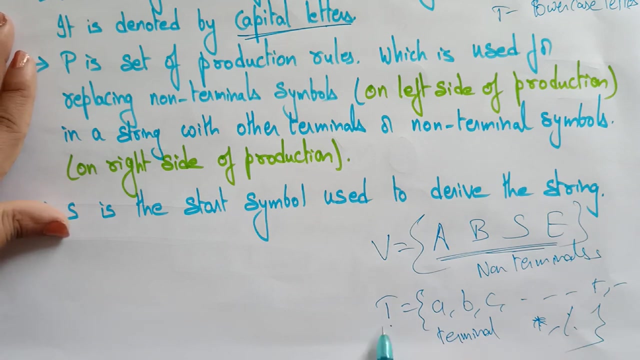 We represent it as V- Non-terminals. And what about the T? T is a terminals. Terminals means A, B, C, So plus, minus into divide. So these are all terminal symbols. Remember that Terminal symbols. This is the main difference between the non-terminal and the terminal. Okay, P is a terminal symbols, V is a non-terminal symbols. And coming to the P, P is a set of production rules. 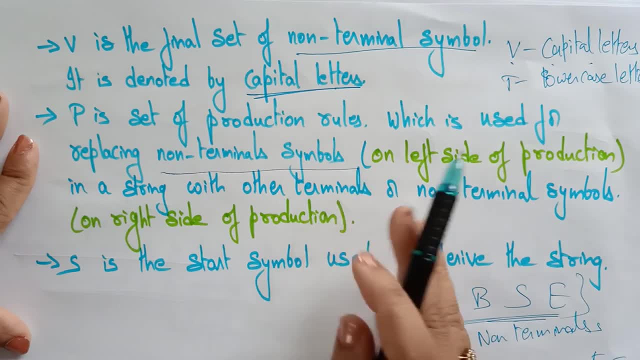 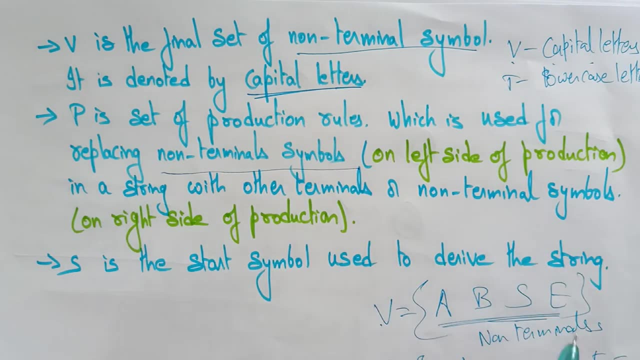 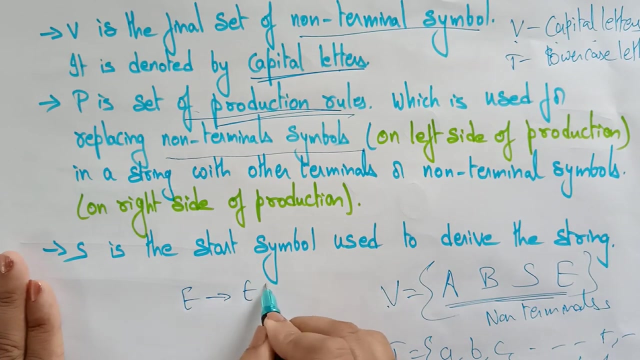 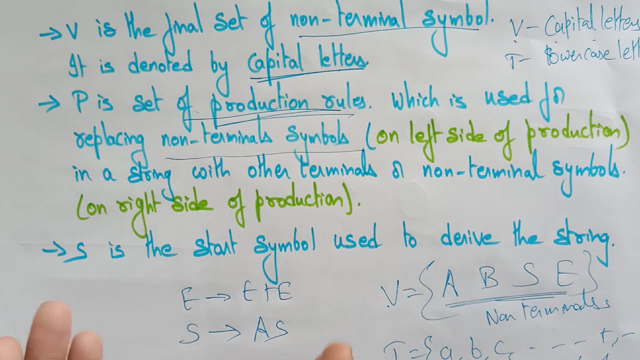 Which is used for replacing non-terminal symbols on left side of the production in a string with other terminals or non-terminals on right side of the production. The one thing that you have to remember that What is a production rule? A production rule means it consisting of: Okay, This is the production rule you call it as Or S determines A- S. So this is a production rule. Or S determines B or A, Okay. 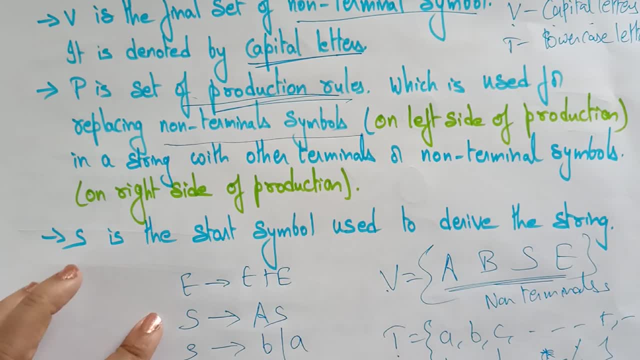 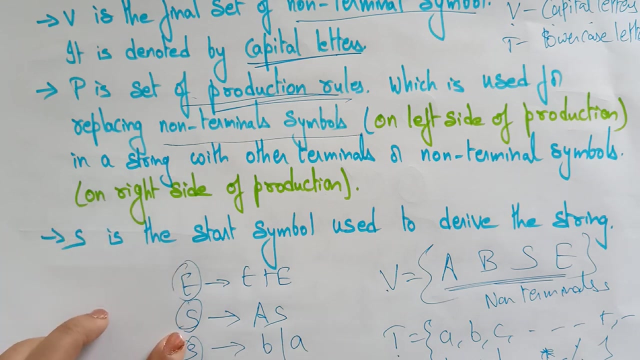 So these are the different ways of representing the production rules. So here a production P is a set of production rules which is used for replacing the non-terminals on left side of the production. So these are the left side, Which you call it as a non-terminals, Because all are capital letters. Whenever these are on the left side, always it is a capital letters. Remember that Left side should be capital letters And the right side should be capital, as well as the lower case letters. 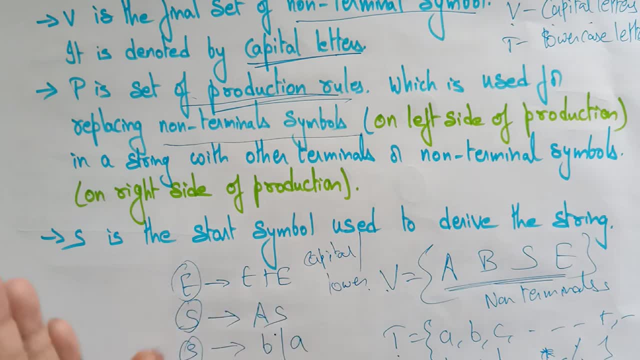 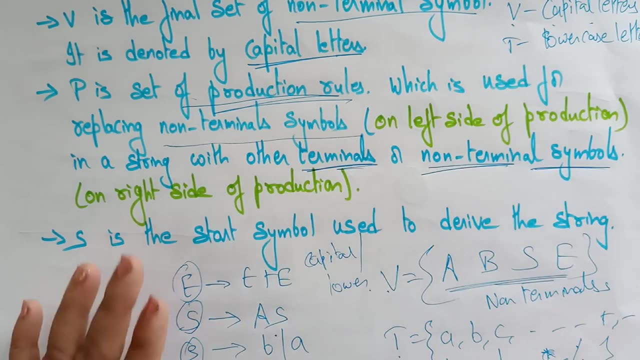 Okay Means this side, in the right hand side, You are having the terminals as well as the non-terminals. Just we talk in the terminology Okay, Or just remove that capital letters and the small letters, Because you have to use the terminology. Remember that terminals means lower case letters, Non-terminals. Non-terminals means the higher case letters, That is, a capital letters. So left hand side is always non-terminals.